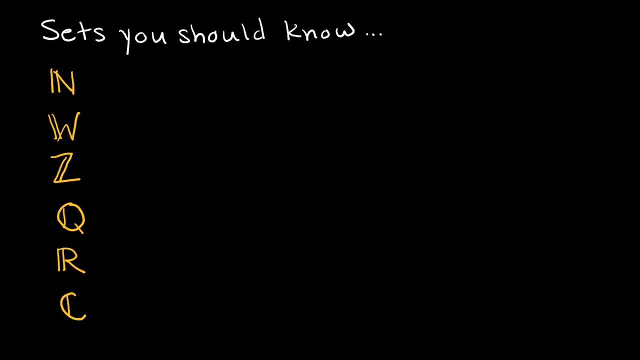 all of these, but I'm going to go through them anyway, just to be safe. So the first set you should know is the set of natural numbers, The set of natural numbers, which means that the set of natural numbers are just the counting numbers. 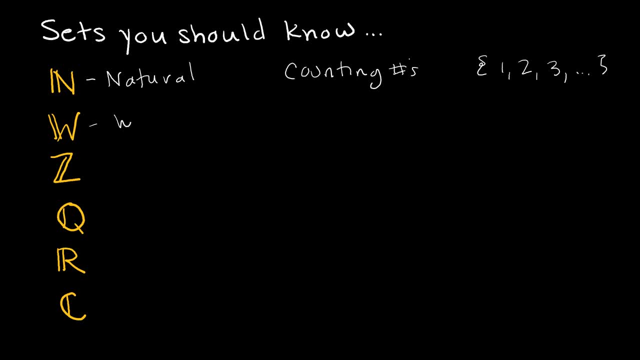 So if I wanted to start listing them, it would be one, two, three onto infinity. W represents whole numbers, and whole numbers are zero, and the natural numbers, which means same set, but starting with zero instead, the integers, And the integers are just the positive and negative whole numbers And of. 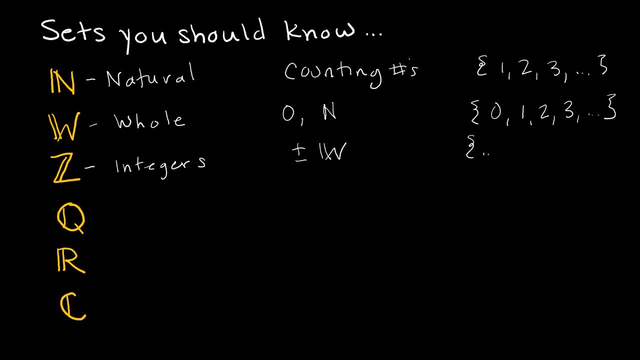 course there is no negative zero, but we get the idea that it would be onto negative infinity. negative two, negative one, zero one, two onto positive infinity. Then we have the rational numbers, which you would think would be an r, but obviously we 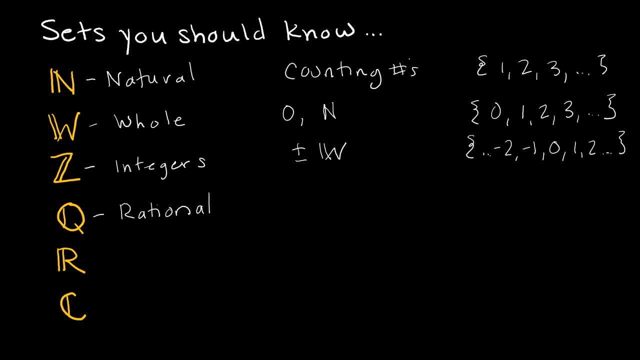 have saved the r for something else. Q represents rational numbers, because a rational number is a quotient of the two terms a and b, where a and b are both integers. B is not zero because of course we cannot divide by zero, And a over b is in lowest terms. 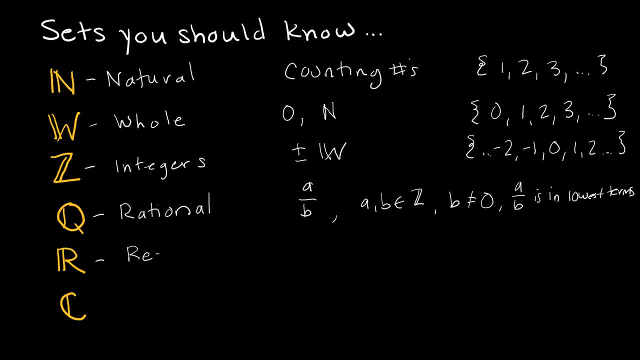 Then we have r, which represents our real numbers, And the real numbers is everything above it. So all the natural, all the whole, all the integers, all the rational, those are all real numbers. So anything that is not imaginary is real. And that brings us to c, which represents our complex numbers, And complex numbers are: 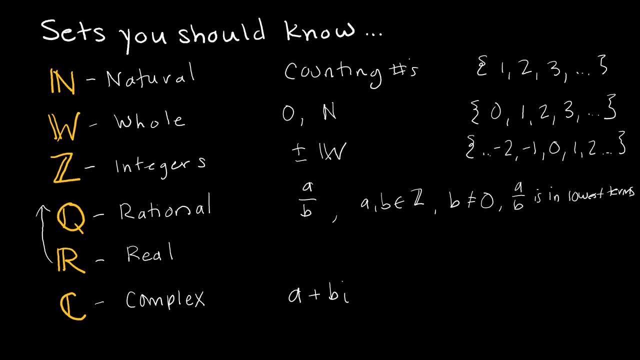 numbers written in the form a plus b i, Where a actually is a real number, It's the real component of a complex number, But, as you can see, b i that i would represent the imaginary portion of that number. So that's all the sets you should. 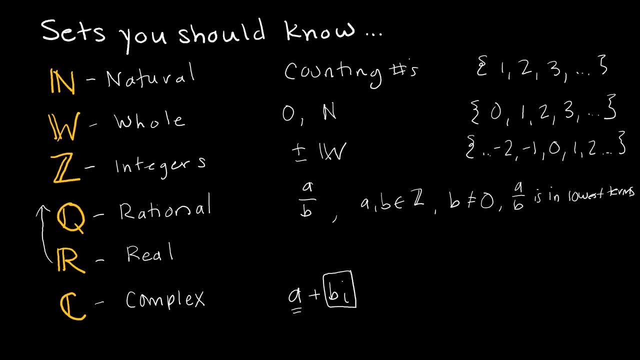 know One more thing I do want to point out. Sometimes you're going to see something like z with a plus or z with a minus, And that would just represent the positive integers. Or if you had negative, it would be the negative integers. 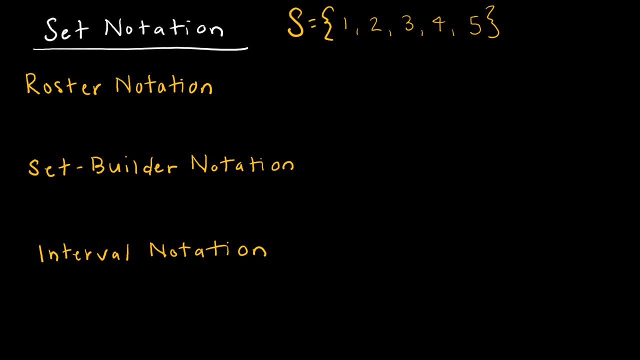 Now let's talk about different types of set notation. So there's roster notation. that is very straightforward. Roster notation, just like the roster of a sports team, is simply listing the elements in the set. So you can see. set s I have said is one, two, three. 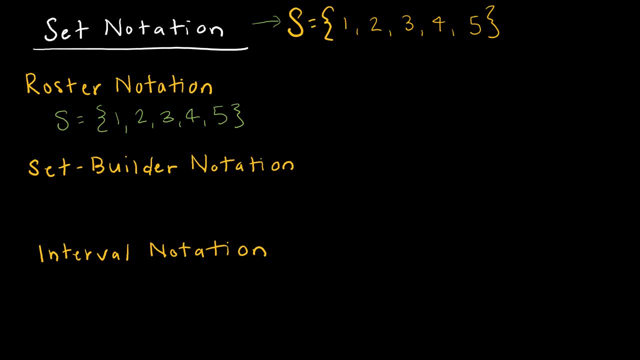 four and five. So roster notation would just be listing the elements in the set. So you can see those roster notation needs to be used with discrete sets. and what do I mean by discrete sets? well, hopefully we know, since here we are in discrete math. 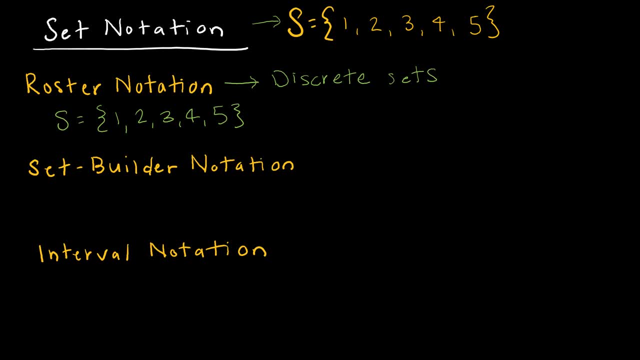 studying discrete objects. discrete sets include things that are countable. they are not continuous. so let me give you an example of something that would be not discrete would be: 0 is less than or equal to. X is less than or equal to 1. if I'm looking at all of the values between 0 and 1, there are quite a few. there are. 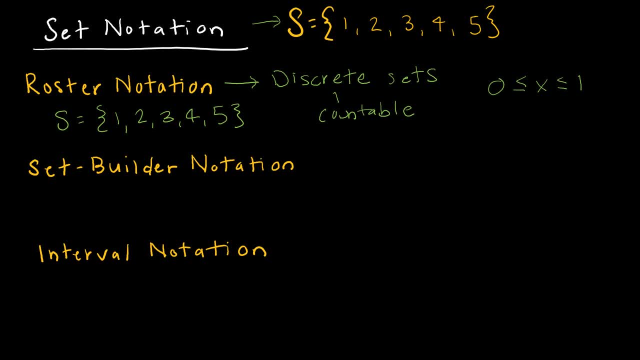 actually infinite number of values between 0 and 1, because they could say 0.1, 0.2, 0.3, 0.4, etc. but then I could say 0.1, 1.2, 1.3, 1. you get the idea I can. 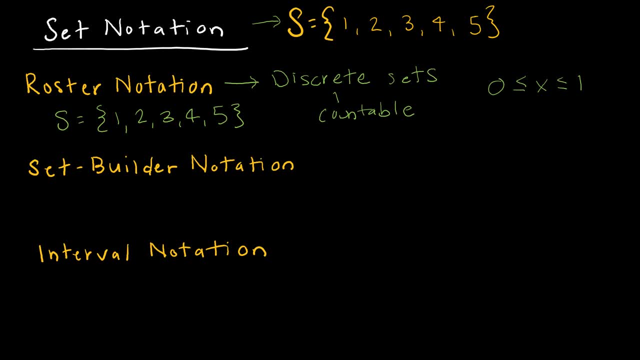 just keep adding another decimal place and that gives me a whole nother you know bunch of numbers that are not discrete. so I can just keep adding numbers that can be included. so this is a continuous set and therefore I cannot use roster notation with that set. has to be a discrete set. then we have set. 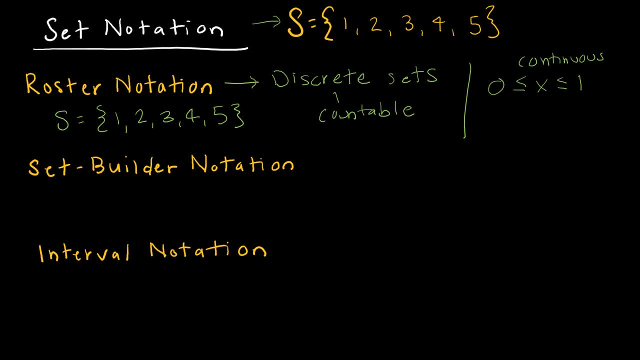 builder notation, now set. builder notation can be used for any kind of set, so it could be a continuous set or it could be a discrete set. so let me show you an example, still using set. 0 is less than or equal to 1 is less than or equal to 1, and that means that set is not. 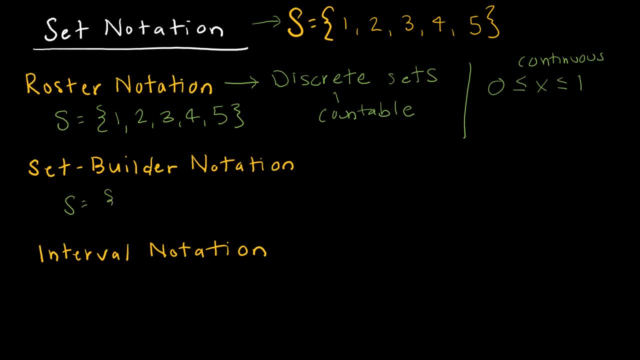 S. if I wanted to write set S in another way, I would say: set S is all of the elements, X, such that. so this little line here just means such that, and everything that follows the such that line is describing the elements in the set. So in this case I could say all of the elements. 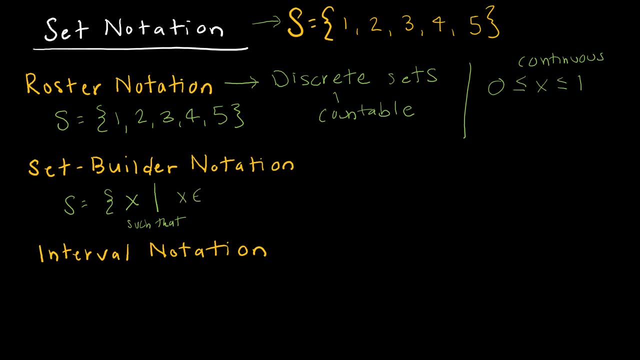 in the set, such that X is an element of the natural numbers- Remember, the natural numbers were just the counting numbers- And also that X is less than or equal to five. Does that describe my set? Well, absolutely it does. It describes my set, but also, I could have 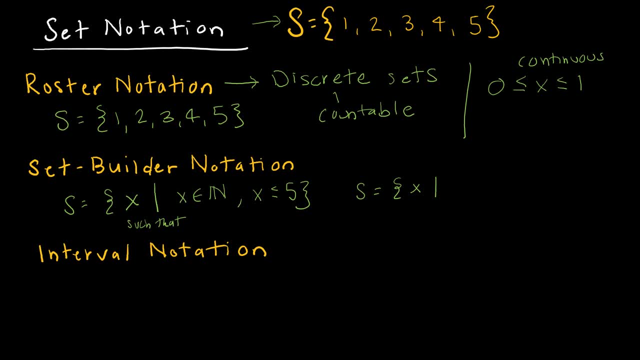 said all of the elements X, such that X is an integer. Well now, integer integers include the negative and positive values. So here I would have to say that zero- I'm sorry one- is less than or equal to X is less than or equal to five. 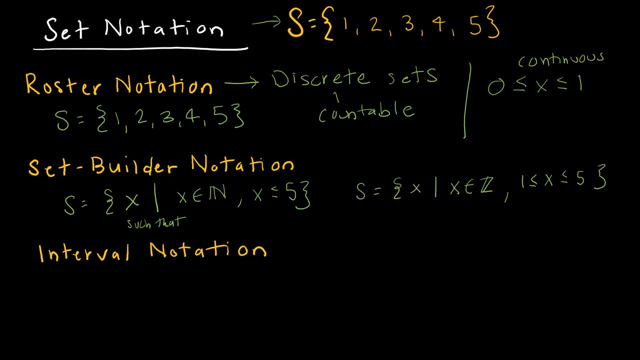 So that's another way to correctly talk about set S in set builder notation. Now let's talk about interval notation. So I'm going to start with set builder notation and we're going to move to interval notation. Let's we have to have a different set. 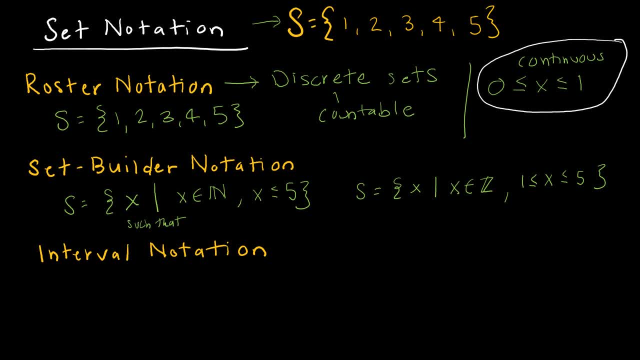 now, because interval notation is what we're going to do with these continuous sets. So we have to use that interval notation or you can use set builder. but most often interval is the best, It's the clearest, it's the easiest. So let's take a look. Let's say set B is equal. 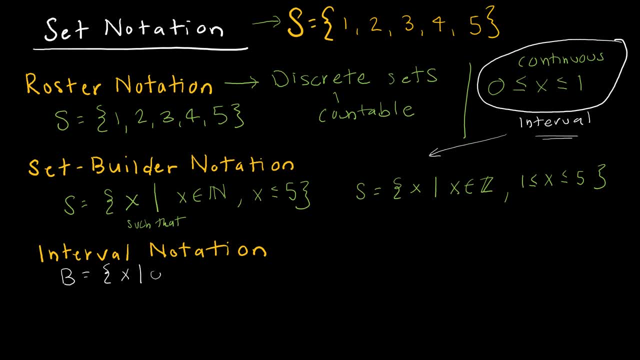 to all of the Xs, such that zero is less than or equal to, X is less than or equal to one. So it's including all of the values between zero and one inclusive. So zero is included and one is included. So if I'm looking at a number line, 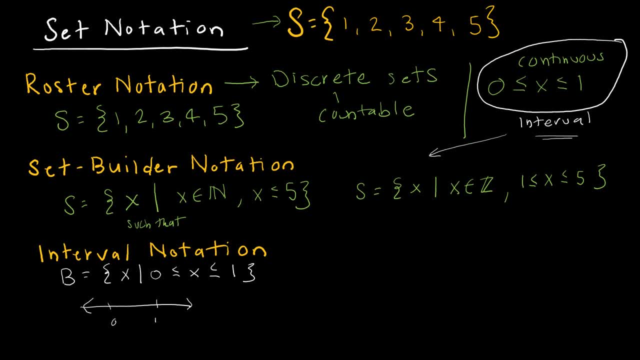 where I have zero and one, and this might bring you back to middle school days. If I were to graph on a number line all of the values that are included in set B, zero would be included, one would be included and all of the values between zero and one are. 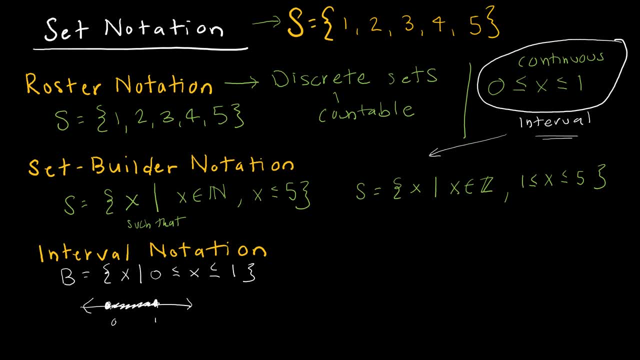 also included. Now, if I want to rewrite this in interval notation, I'm going to pay special attention to the set B and the set B, which are the values between zero and one. So I'm going to Hess to the end points of my interval and whether or not those end points are included. 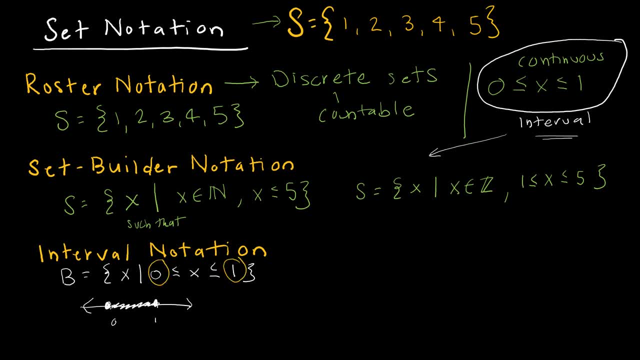 So if I'm looking at the end points, zero and one are the end points, So zero, comma one And interval notation again is only for continuous set, so I don't have to say that it's continuous. Interval notation implies it's continuous. Now 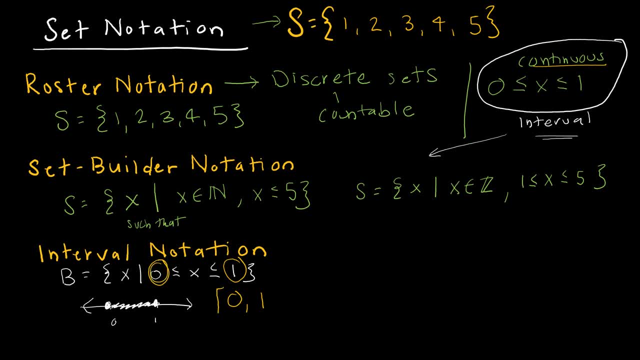 zero is included in this set, so I'm going to use what's called a closed bracket, and one is also included in the set. and again, because these both say or equal to, and so that's how I would write that in interval notation: zero, comma one, with the brackets on the: 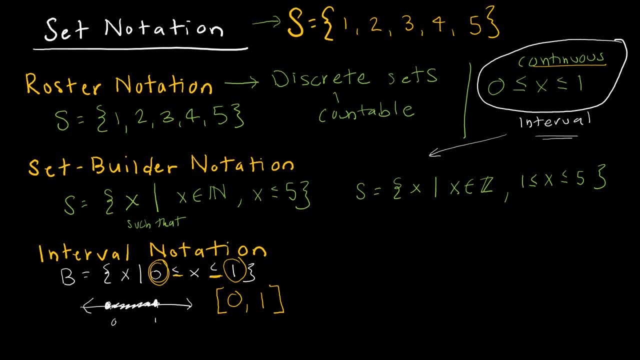 outside, which are closed brackets. Now what if, instead, I said: let's let set m represent all of the x's, such that zero is less than x is less than or equal to one? So what did I change here? Well, I still have zero and one. but now notice: zero is not included, because it's not zero is. 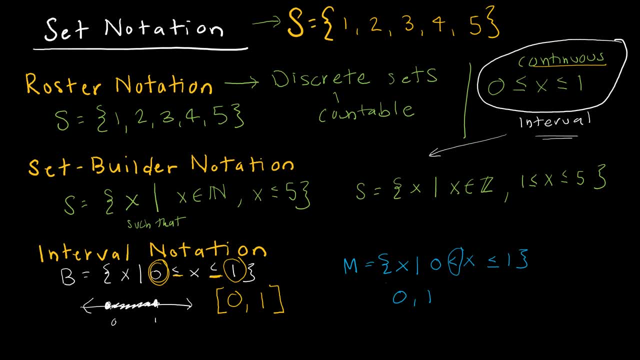 less than or equal to x, which means zero is not included. There we would use an open bracket- Now I've still included the one, so the one would still be closed. or, of course, I could have said that zero is less than x is less than one, and then I would have open brackets on each side. 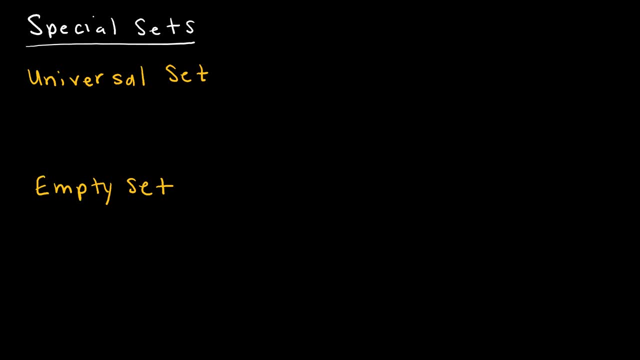 Let's take a look at two special sets. The first is not a term that you're going to hear often, but the concept is important. So the first term or concept is the universal set, and the universal set is essentially the set of all elements, of the set of all elements. 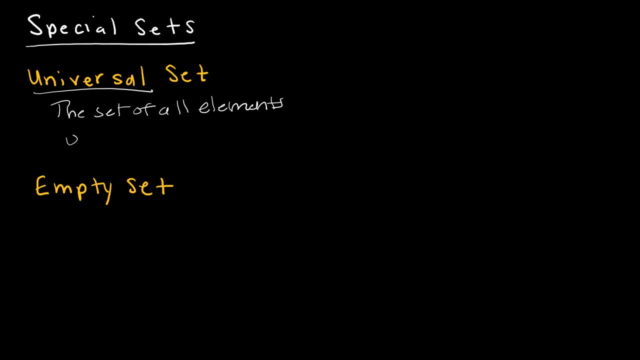 Under consideration, which essentially just means: what am I studying? So let's say, for instance, I was going to create a Venn diagram and I'm interested only in the natural numbers. So this box would represent the universal set of natural numbers. So that's how I would denote that. Now, hopefully,